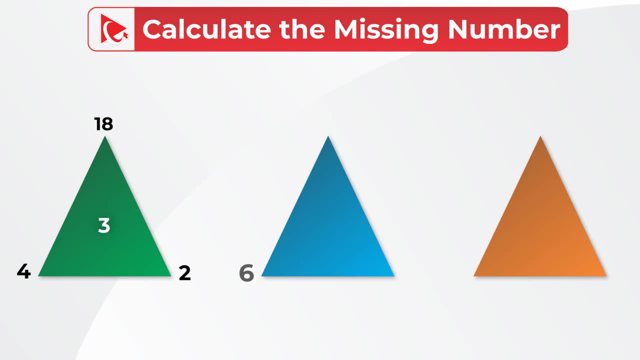 Second triangle has outside numbers 6,, 56, and 1 and has 8 in the middle. And then the third triangle has number 3 in the middle and numbers 5 and 103 on the outside. In the upper right corner of the third triangle you have a missing number which you need to calculate out of four different 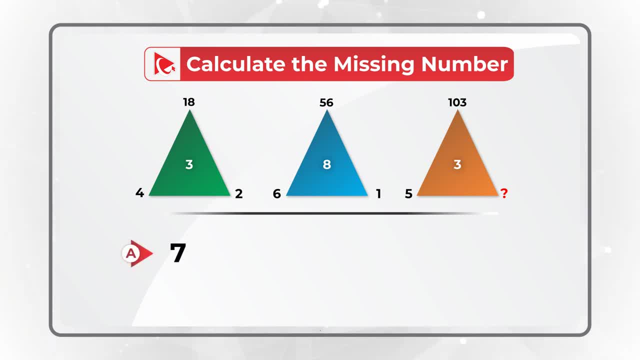 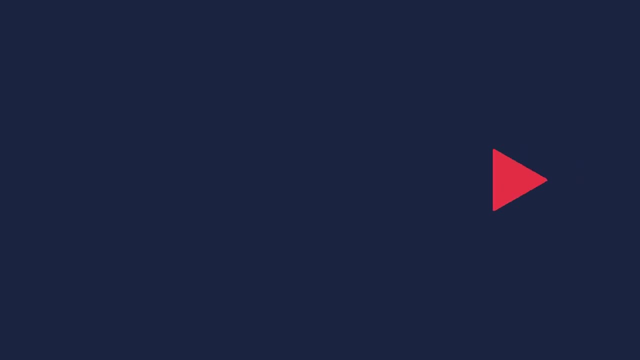 choices: Choices A: 7,, choice B- 10,, choice C- 20, and choice D- 30.. Do you see the answer? The solution is very obvious, but I would like you to try to get to it on your own, Ready or not. I'm moving forward to reveal you the solution, If you have any. 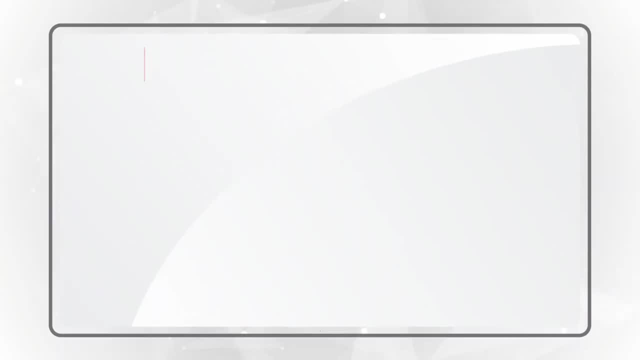 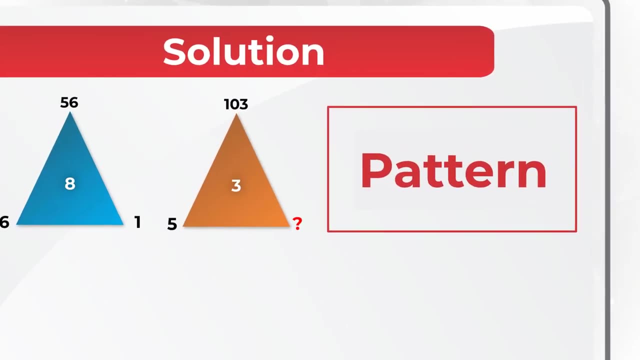 suggestions how to solve these types of challenges faster, please share in comments. One phrase that you hear on this channel the most is always: look for patterns. And then the pattern here is that the top number divided by the sum of the bottom two numbers on the outside of the triangle 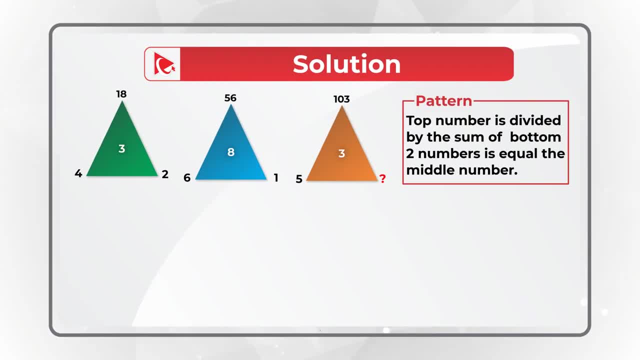 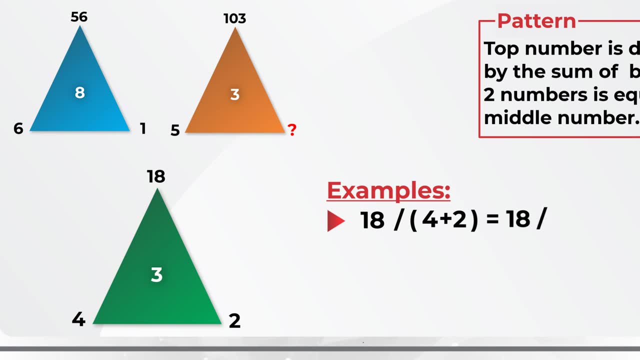 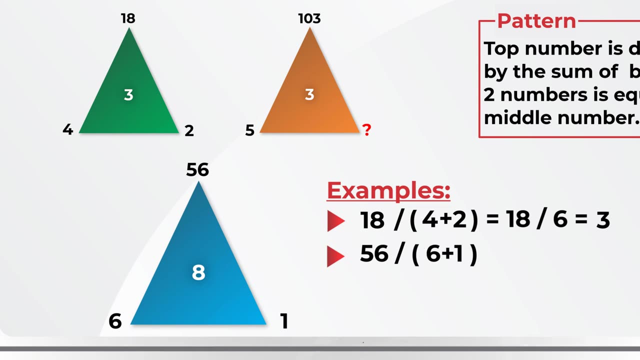 is equal the middle number inside of the triangle. So let's look at the first two examples: 18 divided on 4 plus 2 equals. 18 divided by 6 equals 3.. In the second middle triangle, 56 divided by 6 plus 1 equals 56 divided by 7 and equals 8.. So to calculate the missing number, 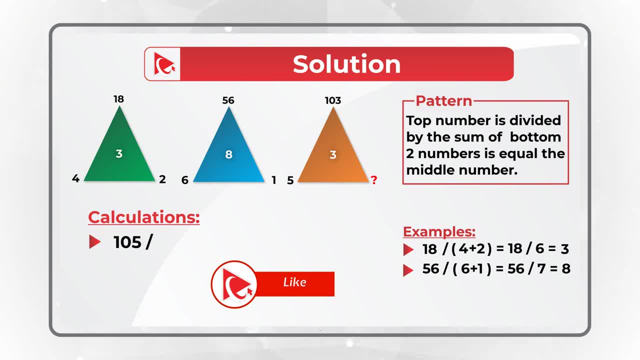 we need to build an equation: 1 of 5 divided 5 plus missing number equals 3.. To calculate missing number, we need to divide 1 of 5 by 3 and subtract 5.. 35 minus 5 equals 30.. 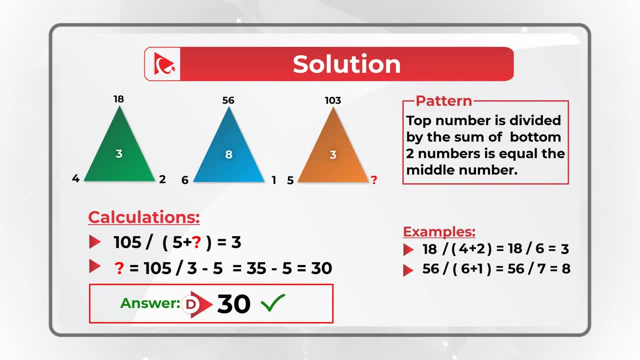 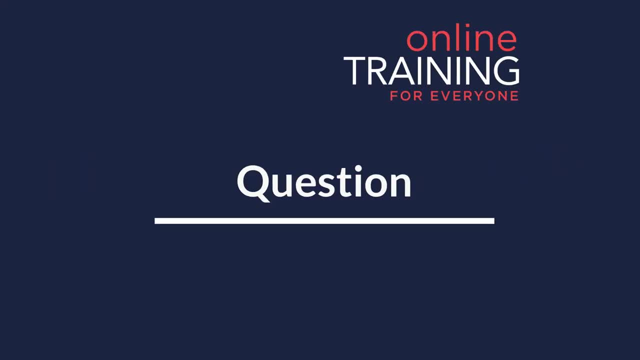 So the answer is choice D 30.. Hopefully you've nailed this question and now can easily solve these types of challenges on the test. I love this question because it truly makes you think. to determine the final answer, You need to determine which number has the lowest value. 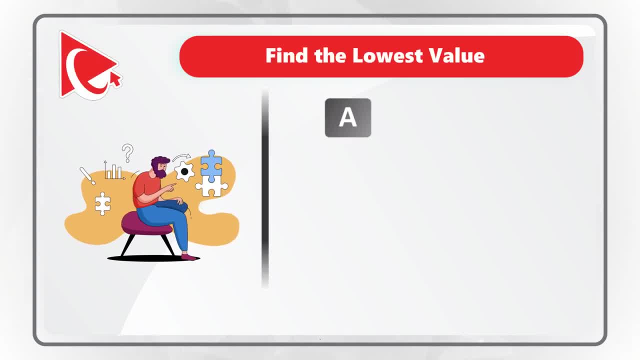 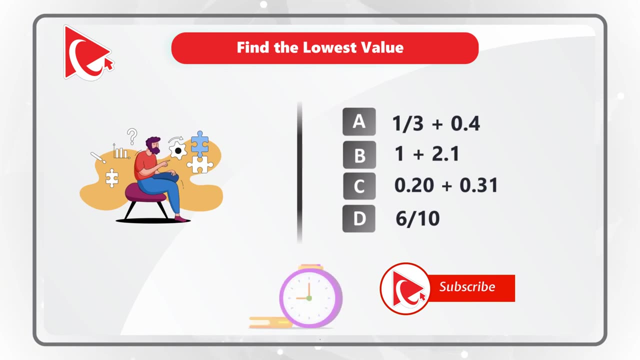 And you have four different choices: Choice A- one-third plus 0.4.. Choice B: one plus 2.1.. Choice C: zero point two plus zero point thirty one. And choice D- six-tenth. Give yourself a few seconds to see if you can come up with the. 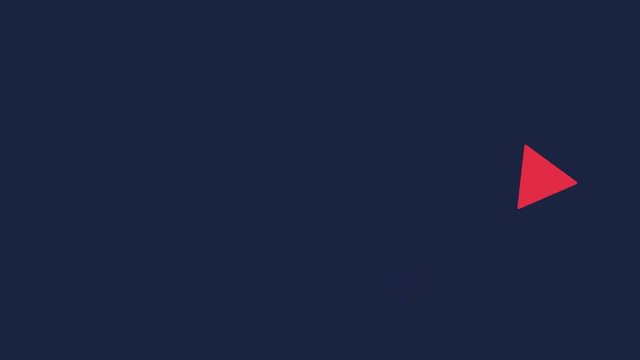 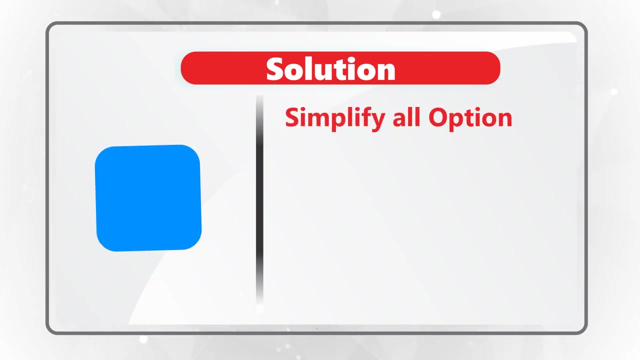 solution. The tricky part here is that the question is designed to make you do a mental math To get to the final answer. you need to simplify all the options. For example, option A: zero point eight plus five is the final answer. Choice B: 0.1 plus 5 equals 5.5 plus 0.3 plus. 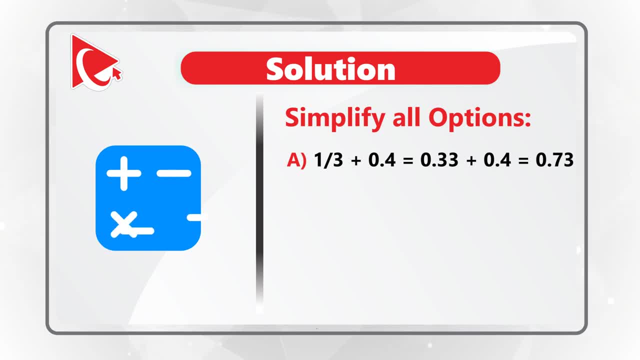 1.4.. Choice C: 1 plus 2.1.. Choice B: 1 plus 2.13 plus 1.31.. Okay, you've gotta solve this. one: 0.4 equals 0.33 plus 0.4, which is 0.73.. Choice B: 1 plus 2.1 equals 3.1.. Choice C: 0.20 plus 0.31. 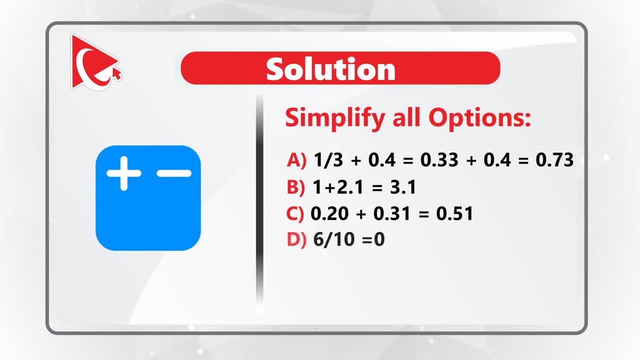 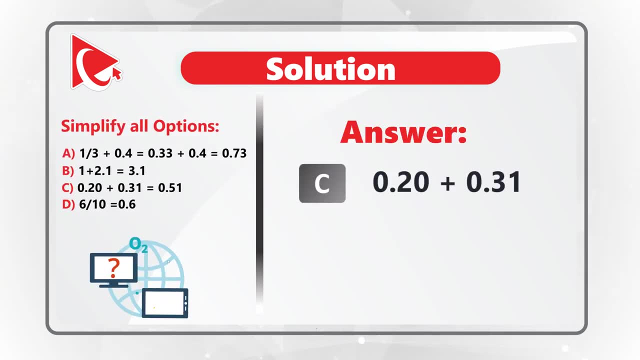 equals 0.51.. And choice D, 6 tenths equals 0.6.. Which means, if you look at the answers, that option C has the smallest value of 0.51, followed by option D, A and B. Was it challenging for you? 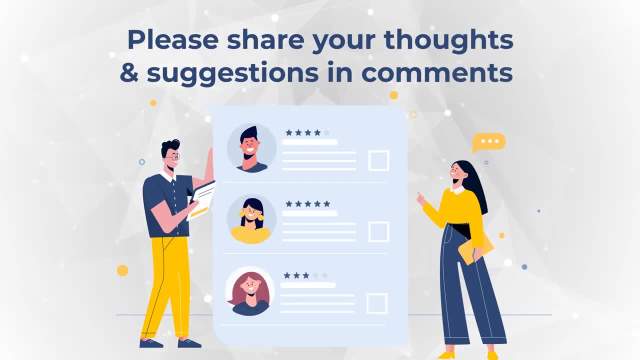 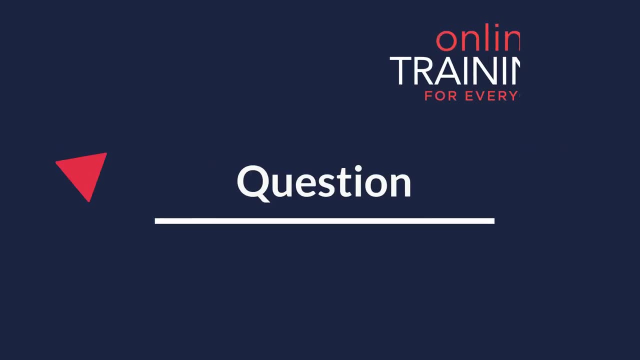 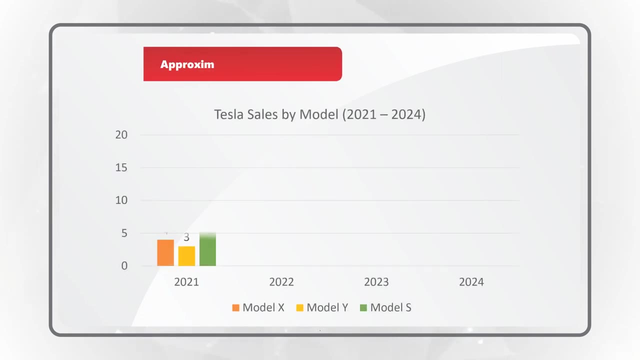 Please share your thoughts and suggestions on how to better solve it in comments. Here is a very interesting question where you need to calculate percentage of Tesla Model S sales in 2023.. You are presented with the bar chart which shows sales for the periods of 2021. 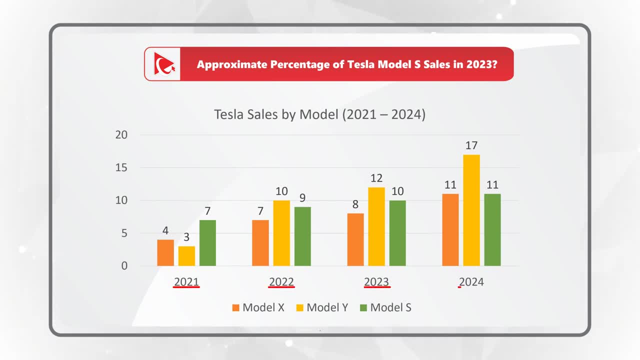 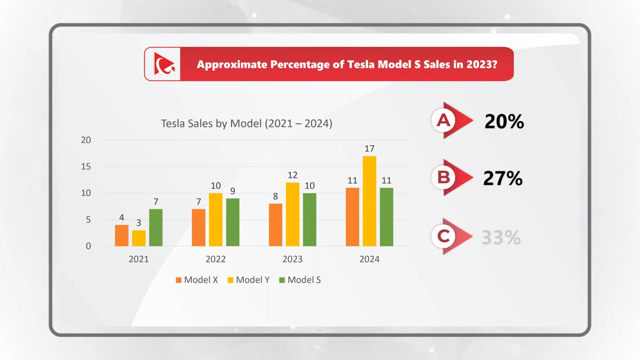 2022,, 2023 and 2024.. And each section has sales for Model X, Model Y and Model S. Based on the information presented, you need to determine which number is correct out of four different choices: Choice A- 20 percent, choice B- 27 percent, choice C- 33 percent and then choice D- 40 percent. Give. 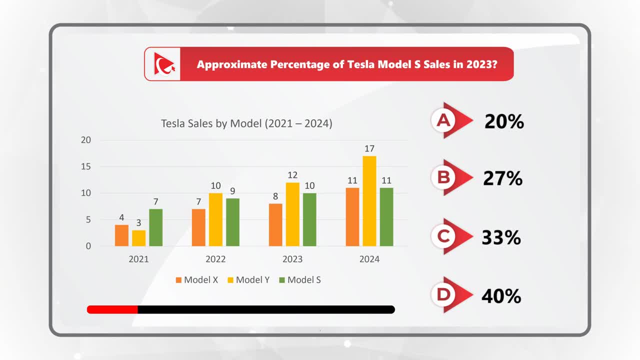 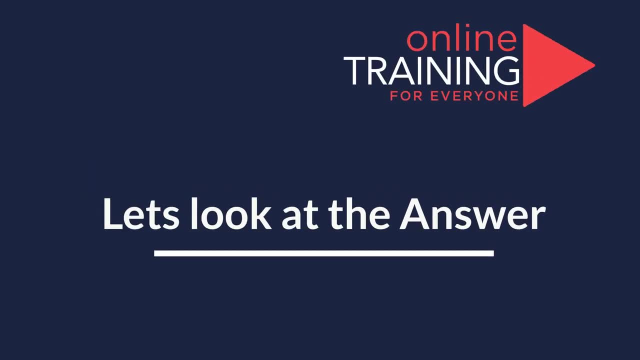 yourself a little bit of time. If you liked this video, please hit the like button. If you have any questions or do you want info on anything, please let us know in the comments. And if you have any questions, please post it in the description. We will be happy to answer them. Hopefully you've figured it out, because I'm 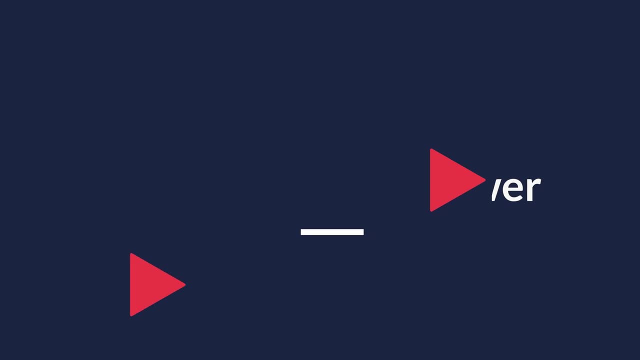 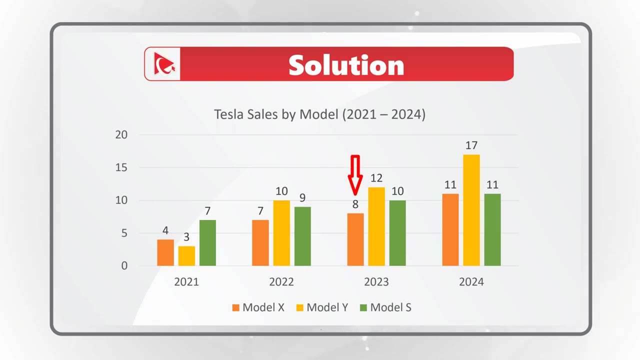 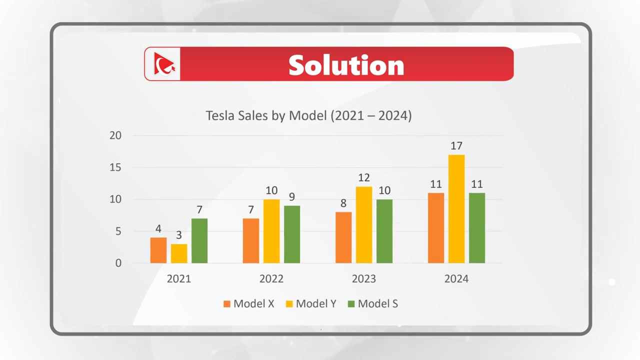 moving forward to share the final answer with you And, obviously, if you have a better way to solve it, please make sure to post in comments. First, let's take a close look at the 2023 sales. You can see that we sold 8 units of Model X, we sold 12 units of Model Y and then 10 units of Model S, so total. 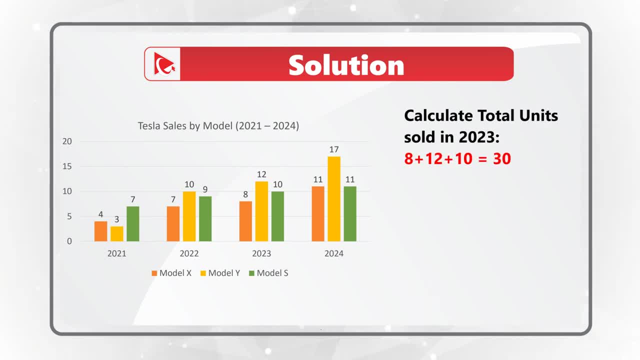 plus 12 plus 10 equals 30.. Now let's determine the percentage. We sold 10 units of Model S in 2023, which is one-third of the 30 units in total. So the correct choice here is one-third of 100%, which is approximately 33%. So the answer here is choice 3, 33%. Hopefully you figured this. 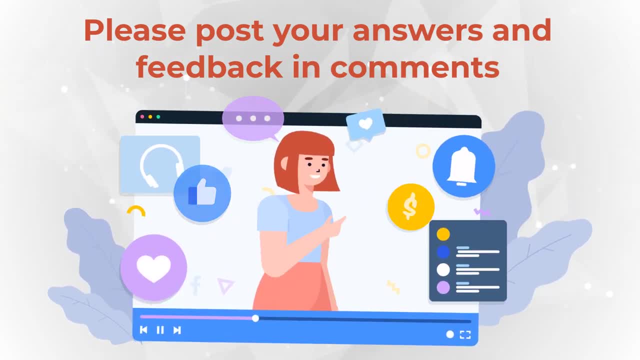 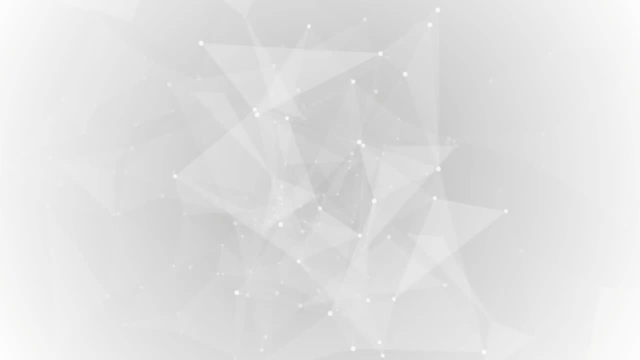 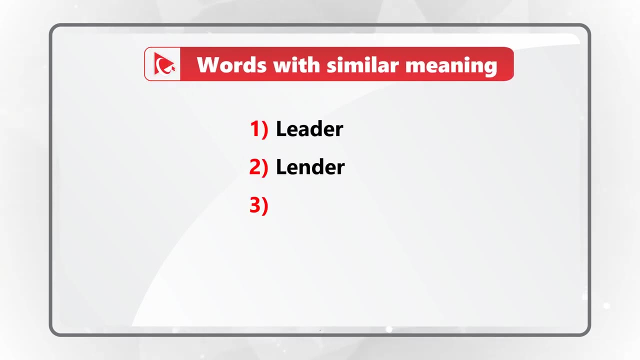 out and now know how to answer similar problems on the test. I love this question because it uses your brain power and also allows you to improve your English vocabulary. You need to identify all the words with the similar meaning. The words are: leader, lender, leather coach and influencer. 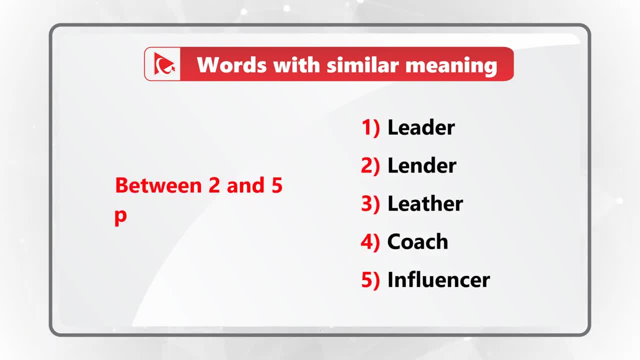 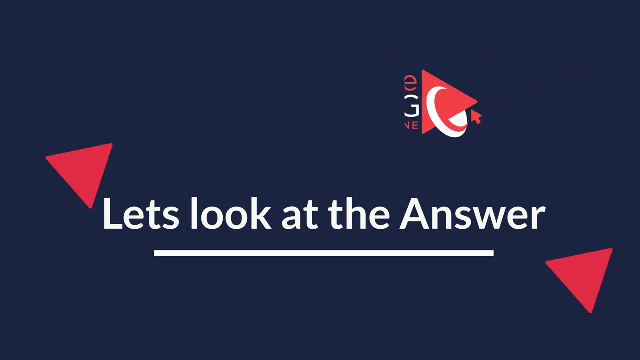 Keep in mind that there could be between two and five words in the answer. What's also interesting is that some words sound similar but in reality represent very different meanings. Ready or not, I'm going to move forward and jump to the solution. Similar words here, as far as I see them, are leader, coach and influencer, And 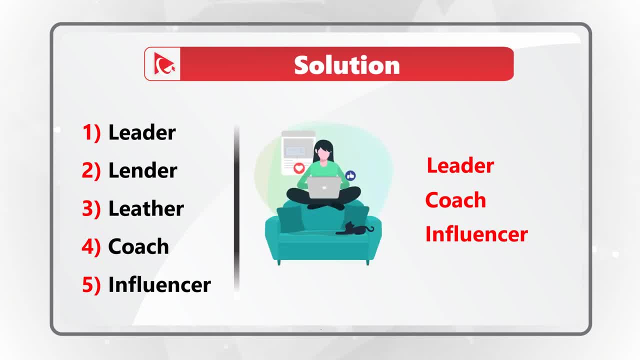 obviously, if you have a different set of words, please make sure to post in comments. Let me share with you why those words are similar. The definition of leader is a person who leads or commands a group, organization or a country. Coach is someone who trains a person or a team. 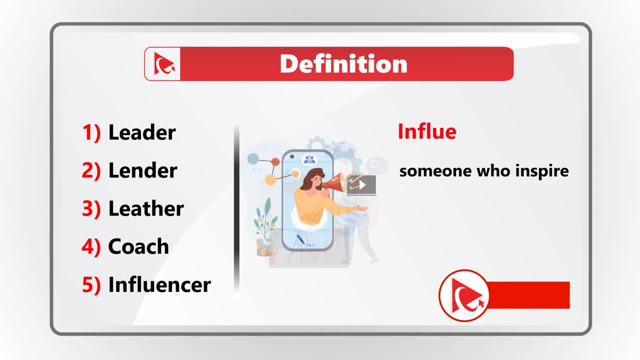 in a particular activity, And an influencer is someone who inspires or guides the actions of others. Basically, the similarity between these words is that they represent someone in power who uses his or her skills to help others. For example, leader could be a. 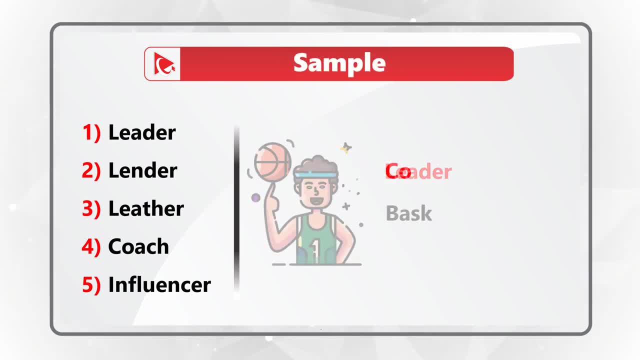 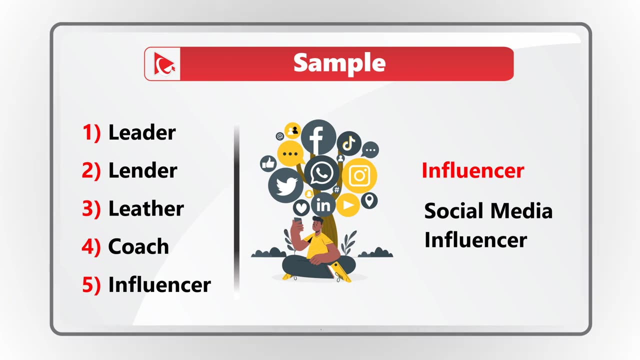 president, prime minister or CEO Coach could be somebody helping with sports activities, like basketball coach, or with personal development, like personal coach. An influencer could be someone who has following on social media, For example, social media influencer. Do you see? 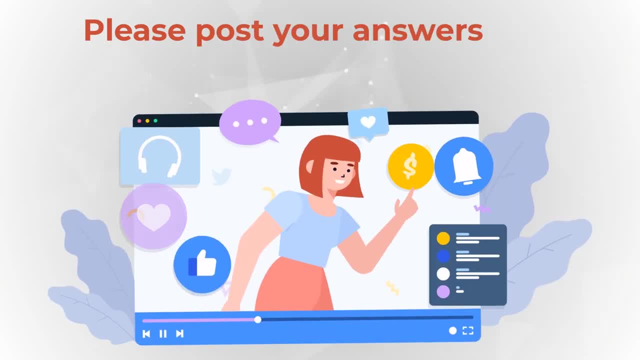 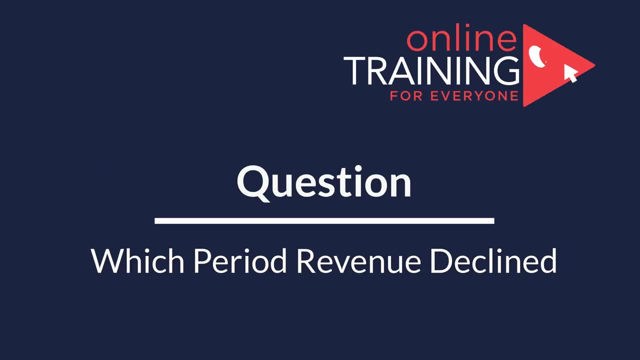 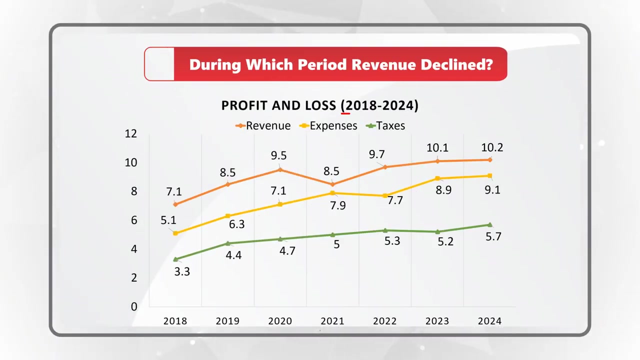 any of these words in the answer. If you have a different set of words, please make sure to post in comments. And now it's time for you to practice your skills to see if you can come up with the answer. You're presented with a chart of profit and loss between the period of 2018 and 2024.. 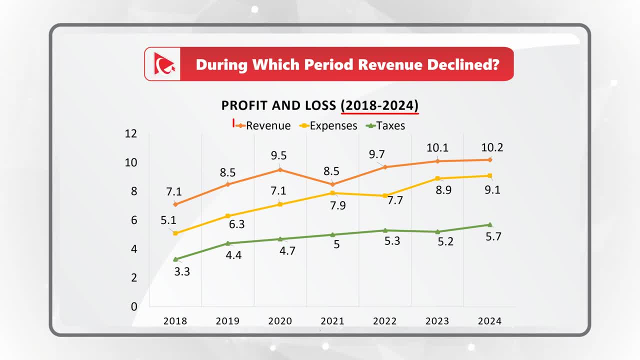 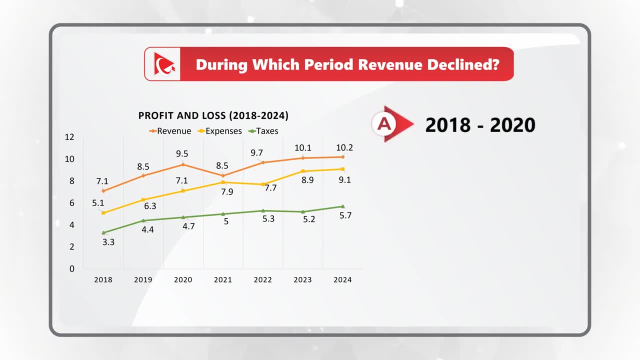 The chart shows revenue, expenses and taxes, And you need to determine during which period revenue declined. You have four different choices to choose: from 2018, to 2020.. Choice B: 2019 to 2020.. Choice C: 2020 to 2021.. And then choice D- 2023 to 2024.. Do you? 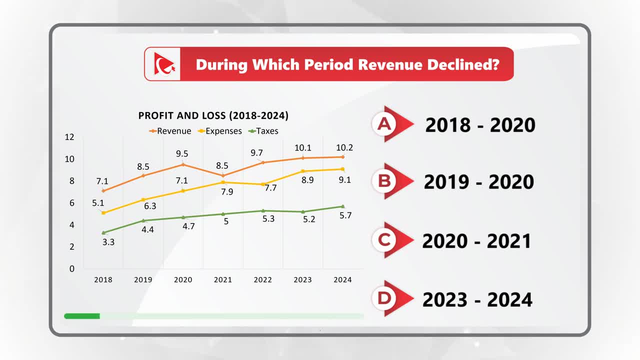 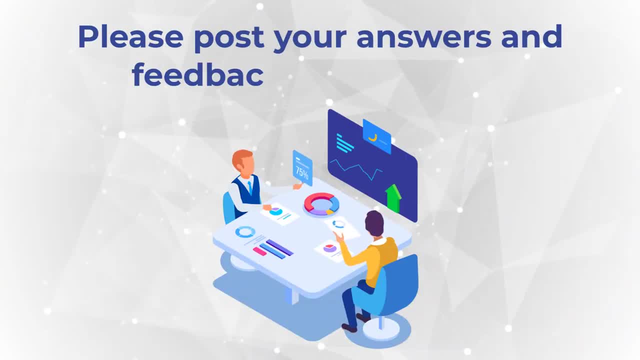 see the answer. I truly hope, with the skills that you learned here, you can quickly identify the answer and post it in the comment section of this video so I can give you my feedback. Thanks for participating and good luck. Very frequently you might get tested on how quickly you can form the. 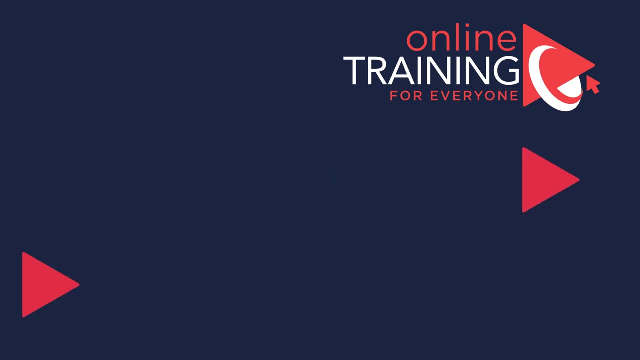 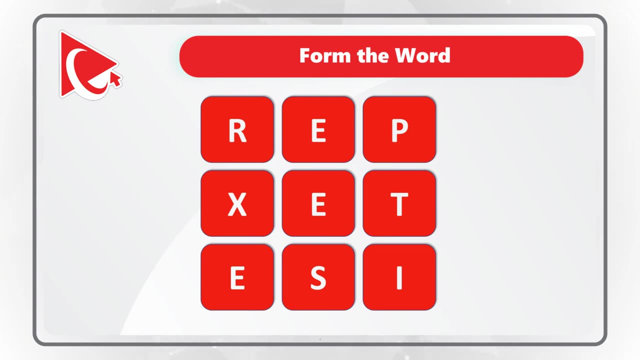 words you want to say. So if you have a different set of words, please make sure to post in the comments section of this video using letters of the English alphabet. In our case, you're presented with nine letters And you need to form the word using all the letters only once The letters are. 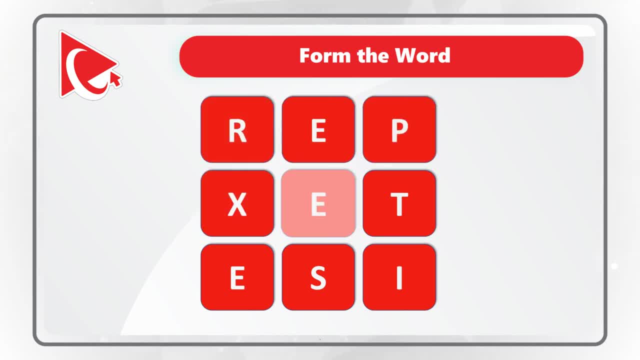 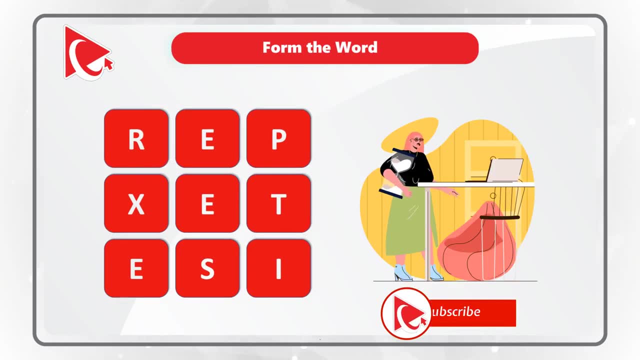 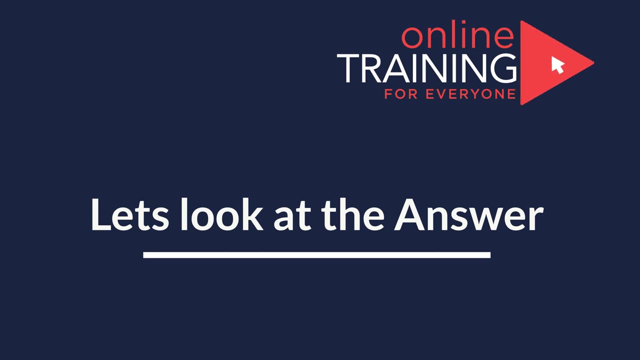 R-E-P-X-E-T-E-S-I. Do you see the word? Give yourself a little bit of time, maybe 10 to 15 seconds, to see if you can answer the question Ready or not. I am going to reveal the answer. 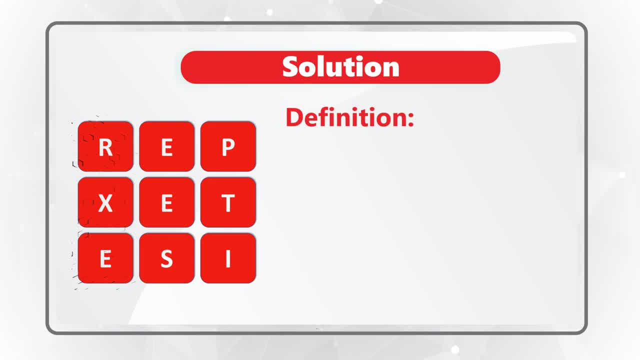 Which is the word expertise, And the definition of expertise is an exceptionally high level of skills, knowledge or performance in a particular task or within a given domain To better solve these types of challenges. try to look at the presented letters and try to form the word. 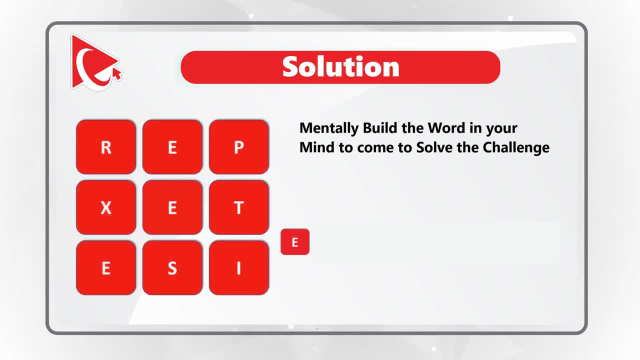 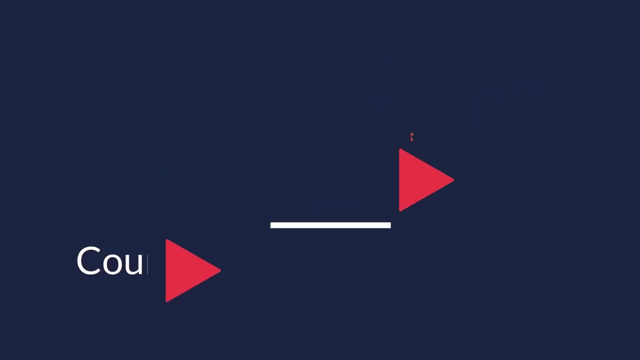 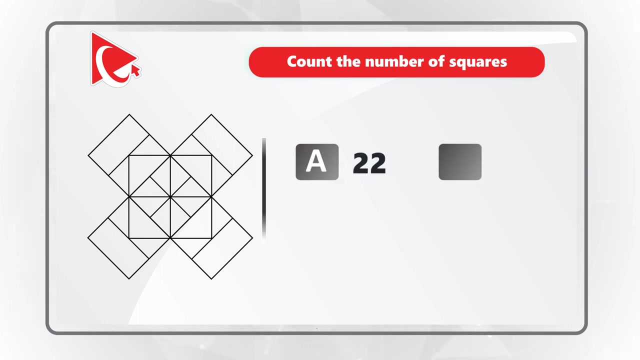 For example, if you start in the middle and go E-X-P-E-R-T-I-S-E, you can definitely form the word expertise. Here is an interesting problem where you need to count the number of squares in the presented shape. The correct number is one of four different choices: Choice A: 22. Choice B: 10. Choice C: 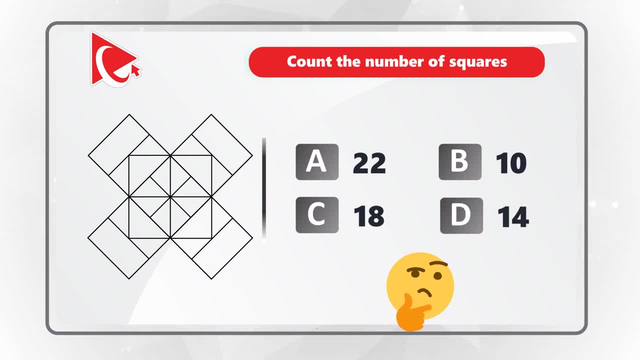 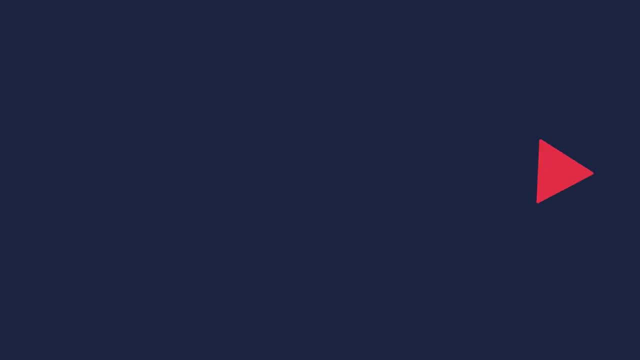 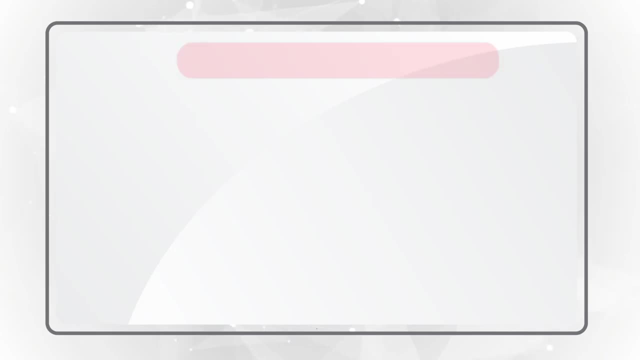 18. And choice D: 14.. Take a close look at the picture to see if you can come up with the right solution. I was really impressed, But there are 18 squares in this picture. Let me show them all to you. 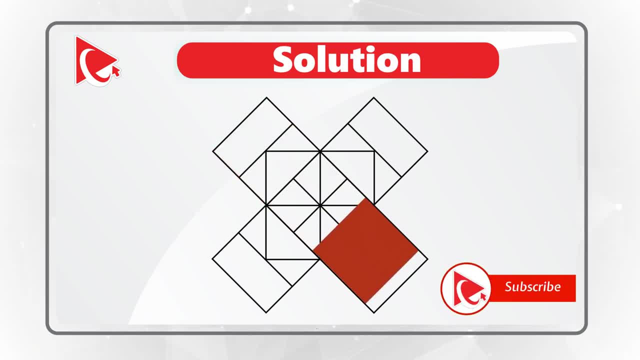 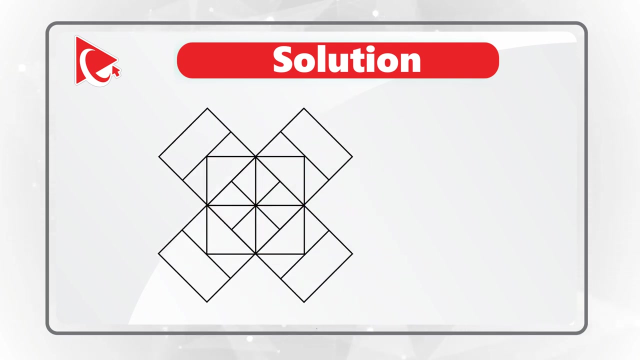 One, two, three, four, five, six, seven, eight, nine, ten, eleven, twelve, fifteen, sixteen, twelve, thirteen, fourteen, fifteen, sixteen, seventeen and eighteen. Do you see any additional ones? It is totally possible that I missed one of the squares. 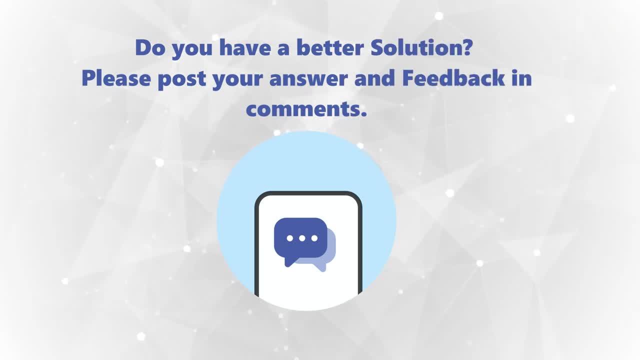 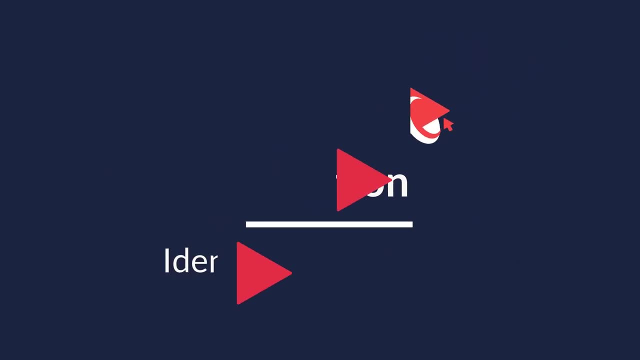 And if you do see any additional ones, please make sure to post them in the comments. I love this question because it seems simple, but it allows you to show all your brainpower. instead of answering it for you, I'd like you to show off and practice your skills. 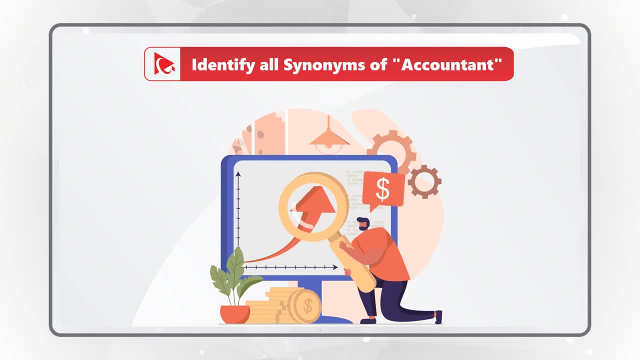 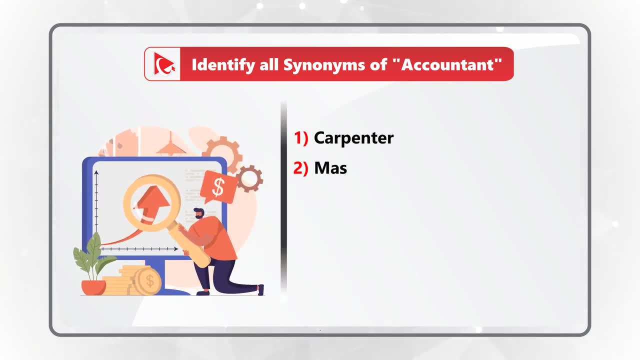 you're presented with ten words and you need to identify all synonyms to the word accountant. ten words are carpenter, Mason, actuary, teacher, auditor, analyst, bookkeeper, engineer, controller and treasurer. question is so cool because there could be between one and ten answers. give yourself a little bit of. 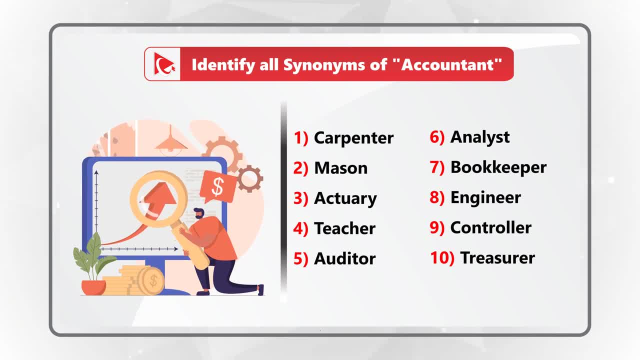 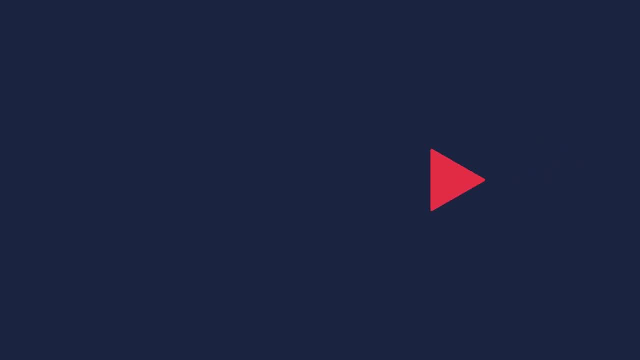 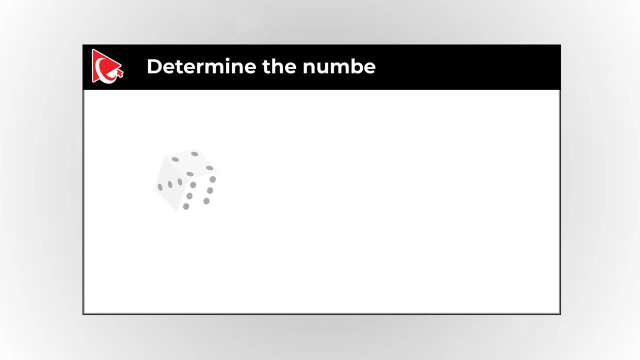 time and when you're ready, please make sure to post your answer in comments. this will allow me to give you feedback. thanks for participating and good luck. here is an interesting question, or you need to determine dice's number at the bottom. dice was rolled twice and dice's numbers have been captured in snapshots. 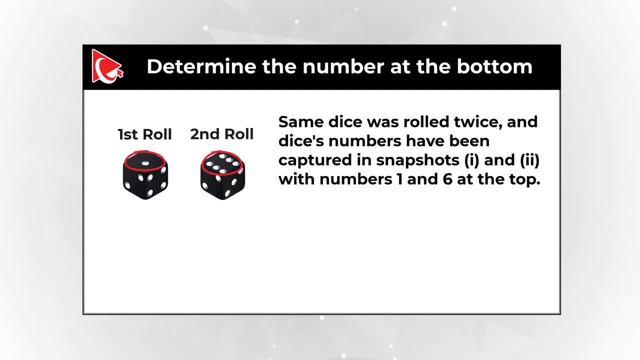 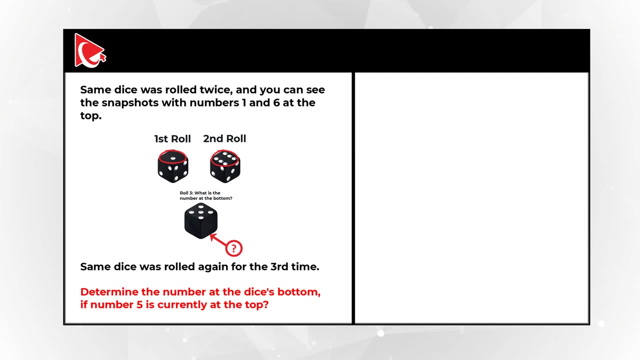 one and two, with numbers one and six at the top you. the dice was rolled again. you need to determine the number at the dice's bottom if number five is currently at the top. you have four different choices: choice a one. choice B two. choice C- three. choice D: six. do you see the answer? please take a. 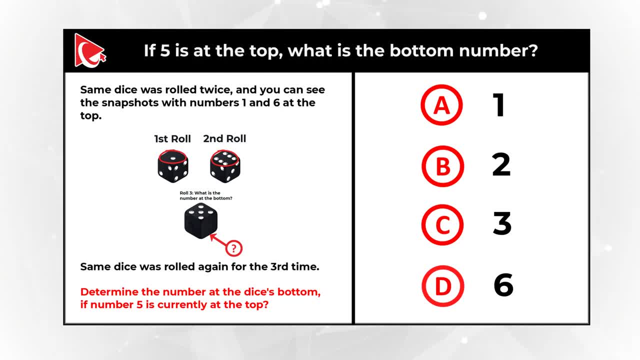 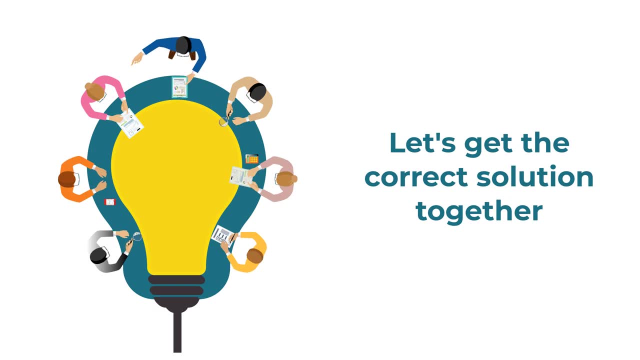 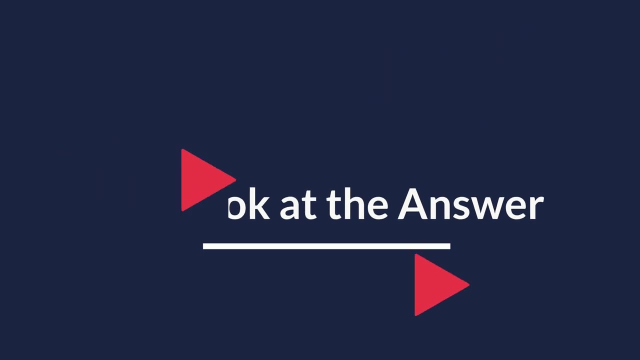 close look because the answer may not be obvious. maybe pause this video to give yourself a little bit of time to find the solution. are you ready? let's move forward and get to the correct solution together to solve this challenge. let's take a close look at the dice. is snapshots based on? 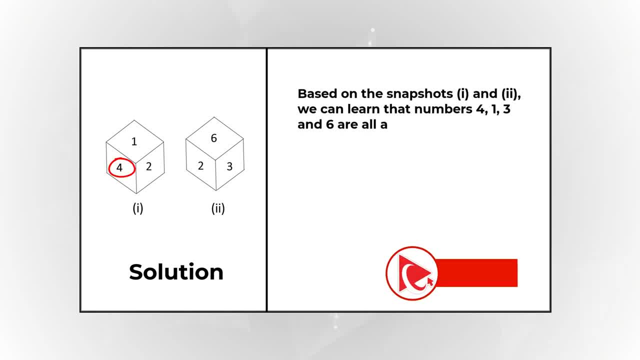 ball snapshots, we can learn that numbers four, one, three and six are all adjacent to number two, because dice are enemies. or is one continent, andrew, a site, and you can go back to the کرmian period and thus help them earn more value from the. 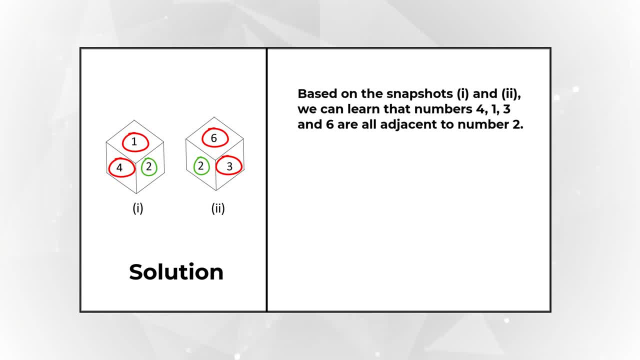 Because dice only has 6 sides and correspondents 6 numbers. based on 2 snapshots, we can determine that 5 must lie opposite of number 2.. This is why if 5 is at the top, then 2 must be at the bottom. 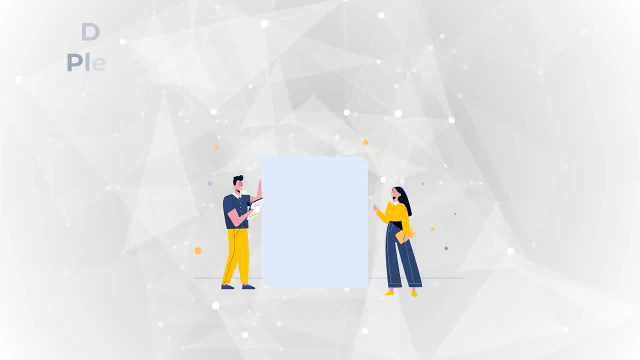 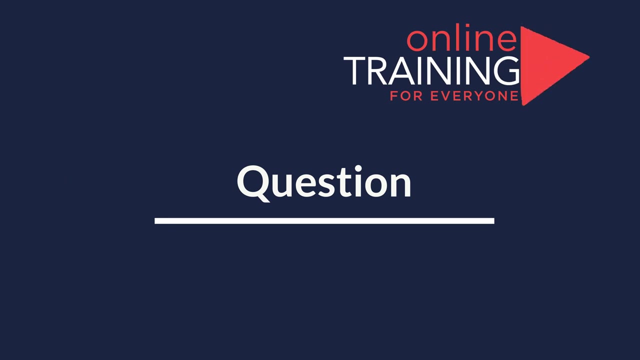 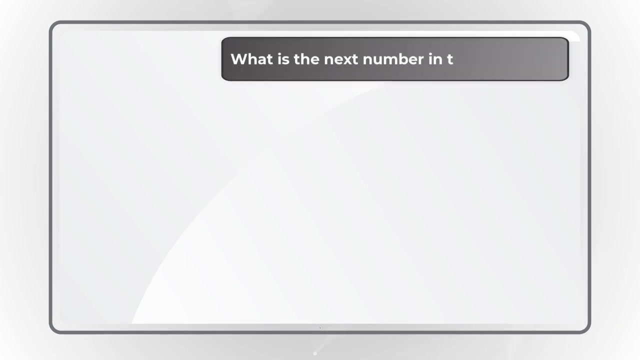 Did you figure it out on your own? Please share your thoughts and the way you solved this challenge in the comment section of this video. Would you like to try your own skills now to see how well you can solve the challenge? This is your opportunity to find the next number in the sequence. 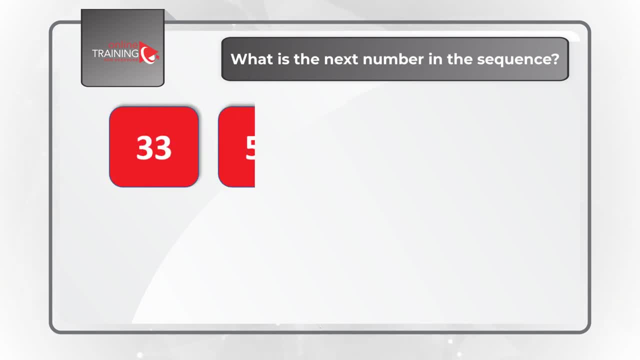 You are presented with 3 different numbers: 33,, 55,, 77, and 1 number is missing. You have 4 different choices to select the solution: Choice A – 97,, choice B – 99,, choice C – 105, and choice D – 107. 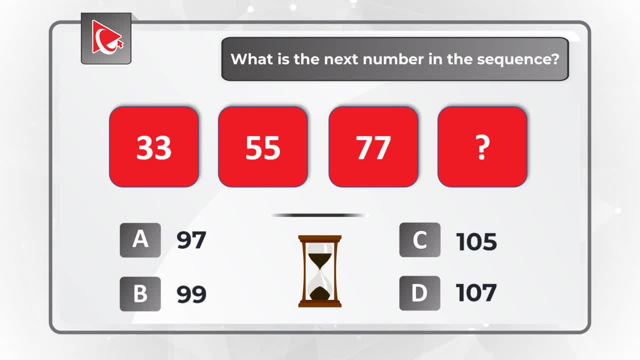 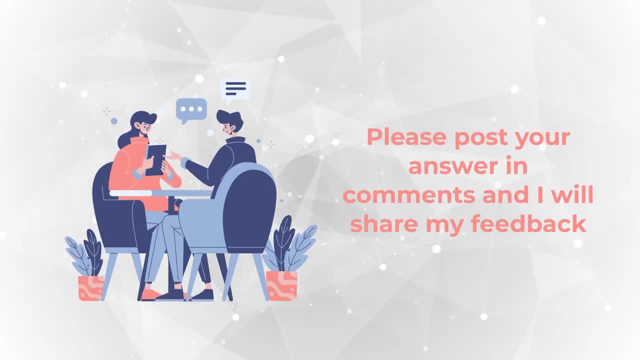 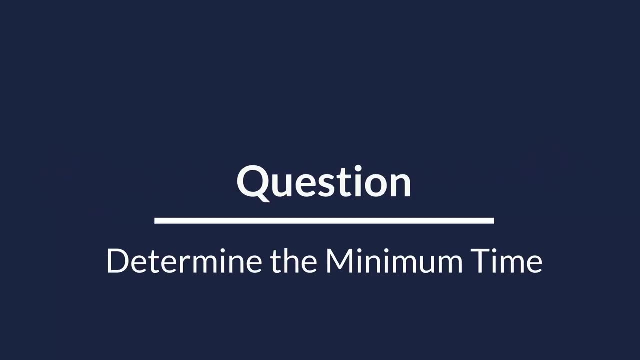 Give yourself a little bit of time to see if you can solve this challenge And once you are ready, make sure to post your answer in comments. This would allow me to give you my feedback. Thanks for participating and good luck. Here is the interesting challenge you might frequently see on the test. 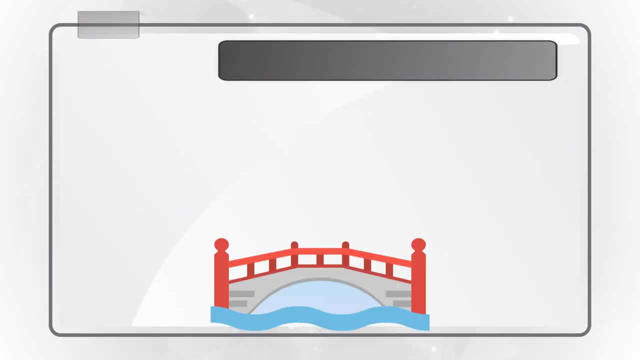 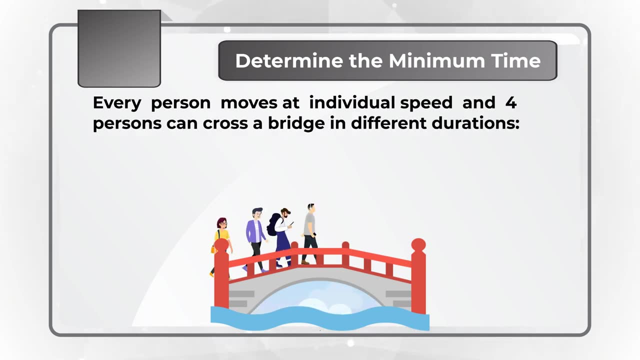 You need to determine minimum time for people to cross the bridge. Every person moves at individual speed and 4 people can cross the bridge in different durations. They can cross it in 3,, 7, 13 and 17 minutes respectively. The trick here is that only 2 people can cross the bridge at the same time. 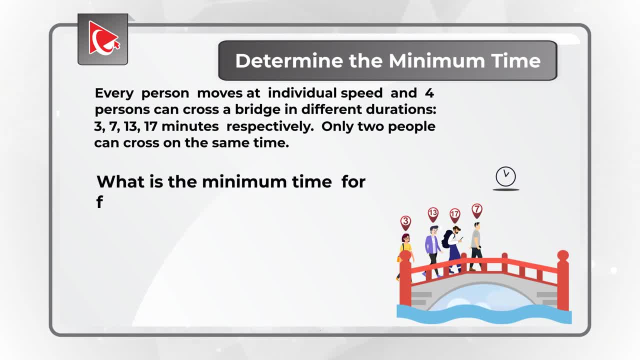 You need to determine what is the minimum time for 4 people to cross the bridge. You are presented with 4 different choices: Choice A – 17 minutes. Choice B – 20 minutes. Choice C – 34 minutes. Choice D – 12 minutes. 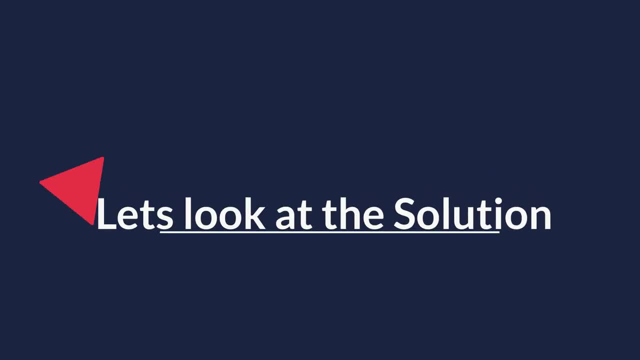 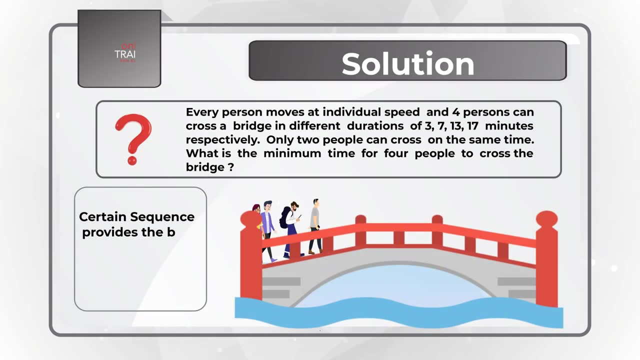 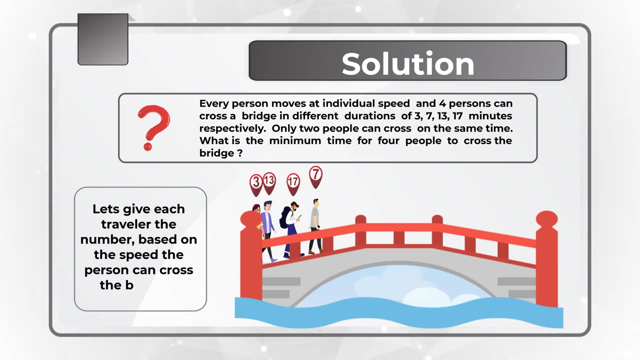 Are you ready for the challenge? Let's move forward and get to the correct solution together. As you might have determined, certain sequence provides the best efficiency for travelers to cross the bridge. Let's give each traveler the number Based on the speed this person can cross the bridge. 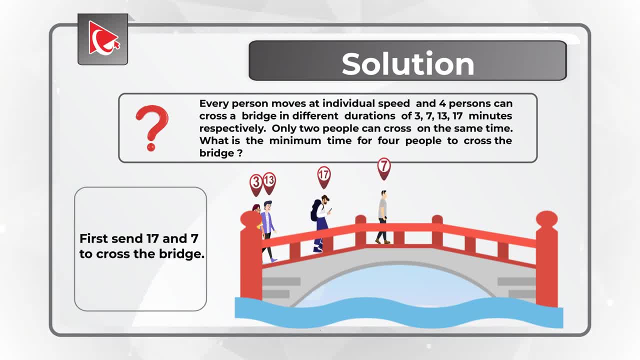 We will first send number 17 and 7 at the same time to cross the bridge. After 7 minutes, number 7 finished crossing the bridge And number 17 needs additional 10 minutes to complete the travel. Let's now send number 13.. 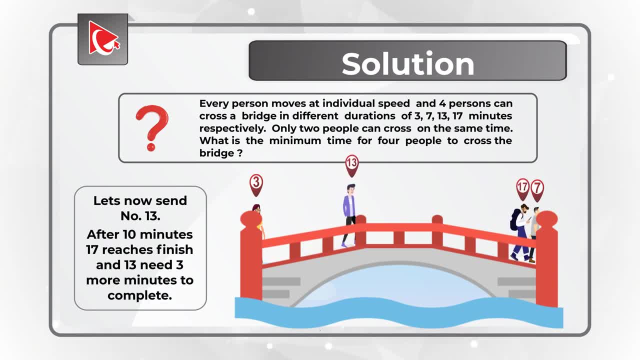 After additional 10 minutes, number 17 reaches the finish line and number 13 needs 3 more minutes to complete the travel. Let's now send number 3.. Both number 3 and number 13 reach the finish line And number 13 needs 3 more minutes to complete the travel. 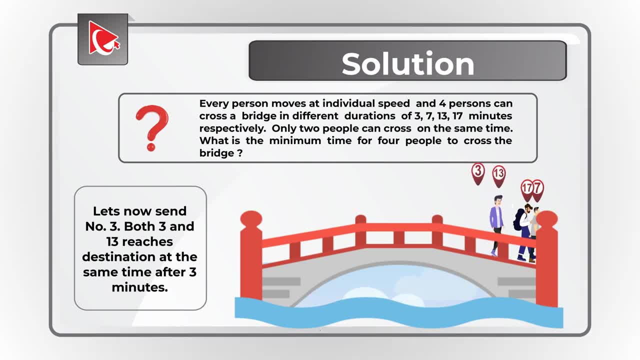 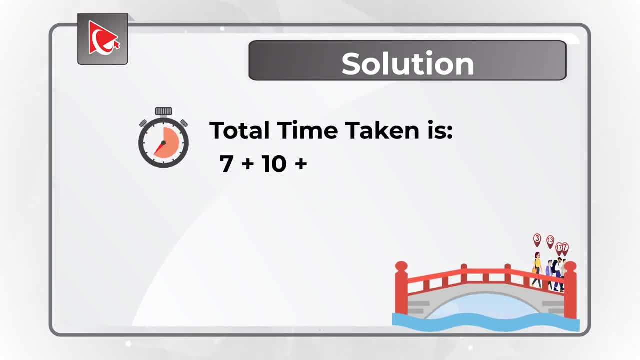 They reach destination at the same time after additional 3 minutes, And total time it took for travelers to cross the bridge would be 7 plus 10 plus 3 equals 20 minutes. So the correct answer here is choice B – 20 minutes. 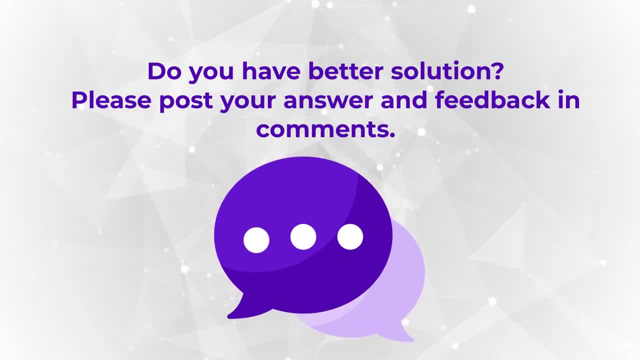 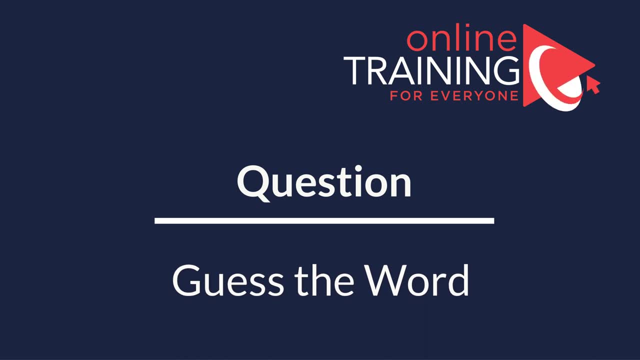 Hopefully you've nailed this question and now know how to answer similar problems on the test. Here's the cool question that you frequently get on the test: You're presented with 4 different letters And you need to guess the word using all letters presented. 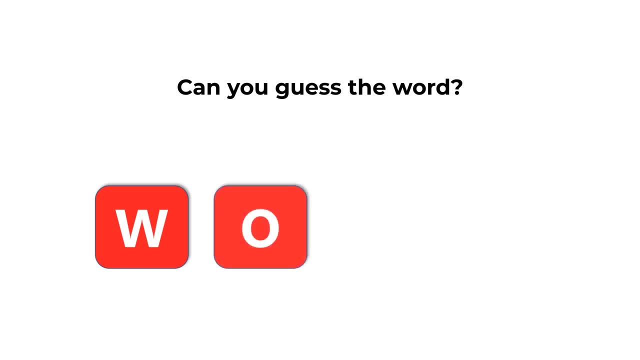 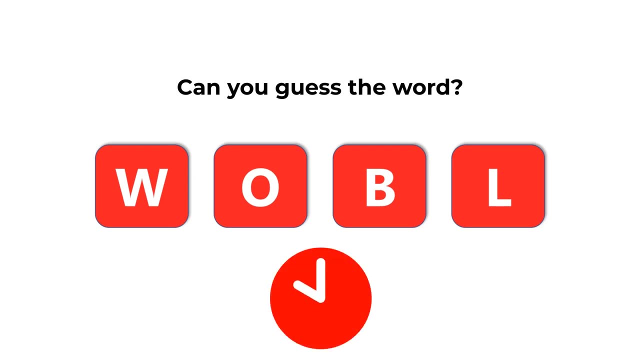 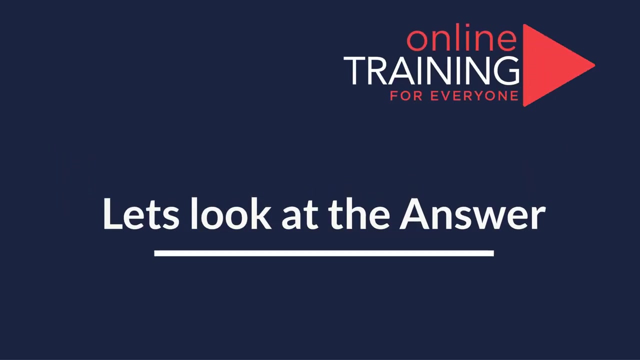 The letters we have are W, O, B and L. Can you guess the word? Give yourself 10 to 15 seconds to see if you can come up with the answer. Ready or not, let's go ahead and reveal the solution. 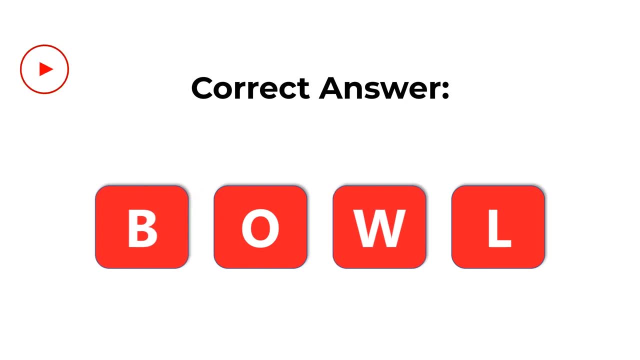 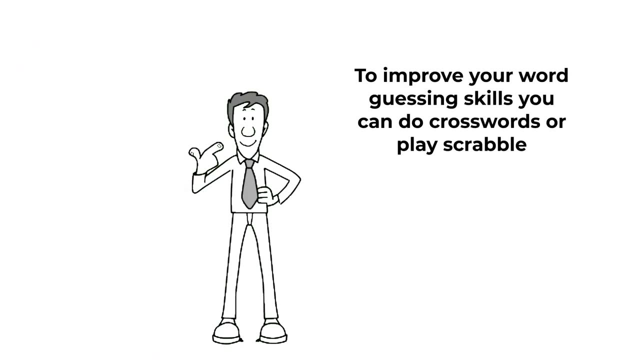 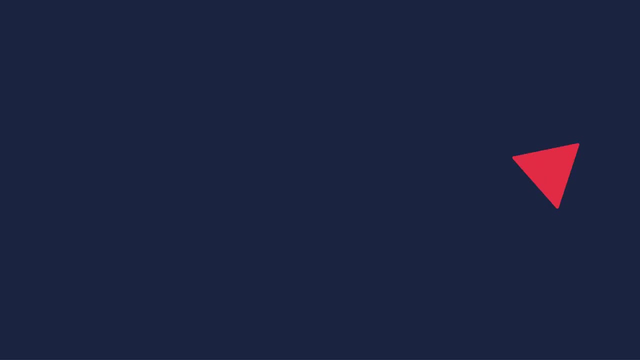 The correct answer here is ball Ball Ball, Which is spelled as B, O, W and L. Hopefully you've nailed this question and now know how to answer similar problems on the test. Let's look at the interesting question where you need to form the word. 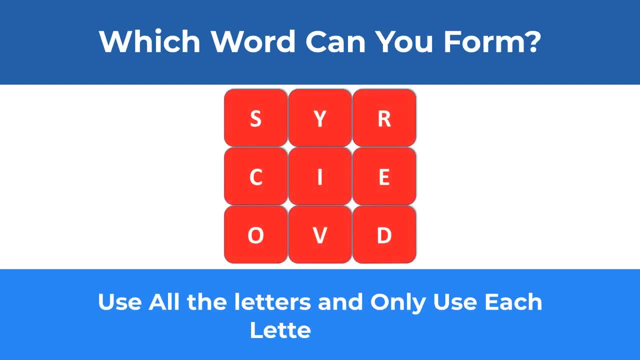 And you need to use all the letters and only use each letter once You're presented with 9 letters. Those 9 letters are S, D and E. The correct answer is Y, R, C, I, E, O, V, D. 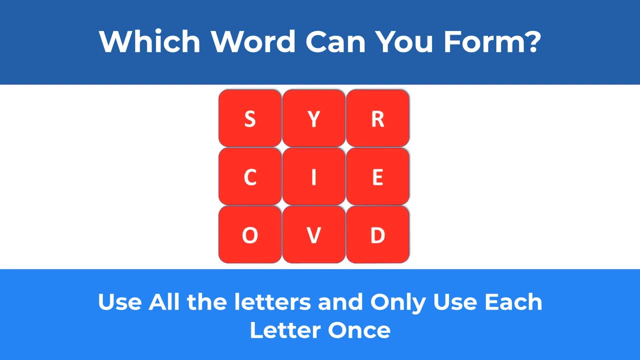 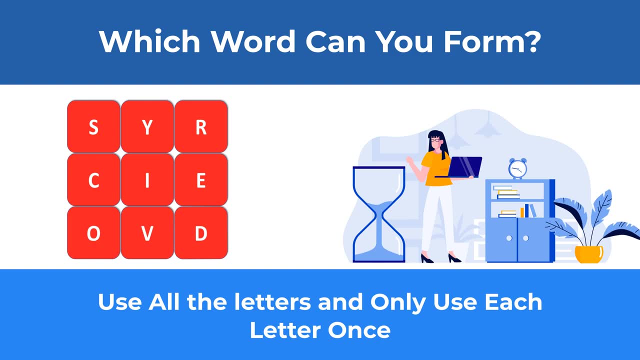 And you need to form the word using all the letters. Do you see the solution? Give yourself a little bit of time, Maybe 10 to 20 seconds. This is typically as much time as you get on a real test, Ready or not. I'm going to reveal you my version of the solution. 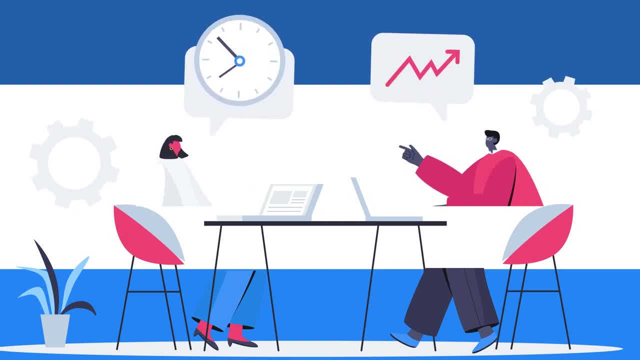 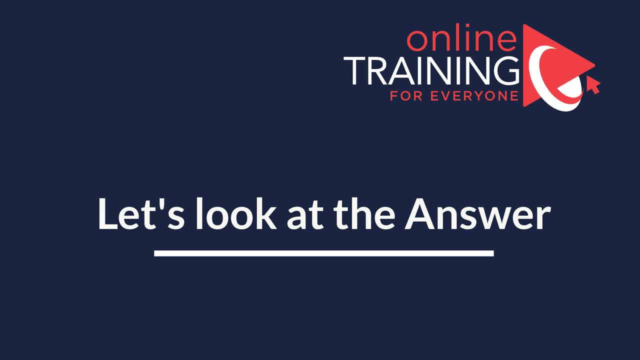 But my version may not be the only one, So if you see other possible options, please make sure to share this video with your friends. See you in the next video. Bye, The word you can form is discovery. Let me spell it for you. 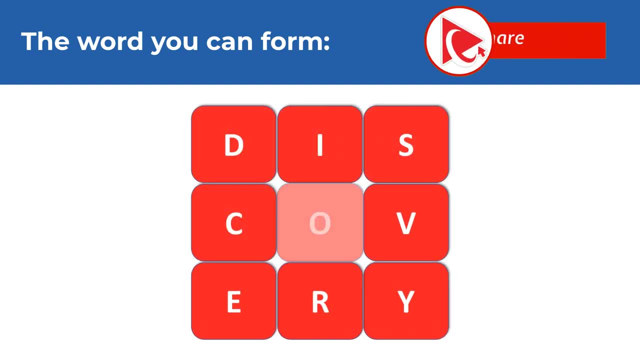 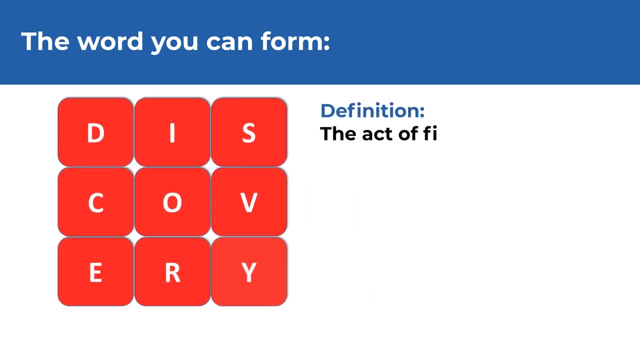 D-I-S-C-O-V-E-R-Y, And the definition of discovery is the act of finding out or learning about something for the first time. Here is the sample sentence where word discovery is used. Scientists consider detection of gravitation as the act of finding out or learning about. 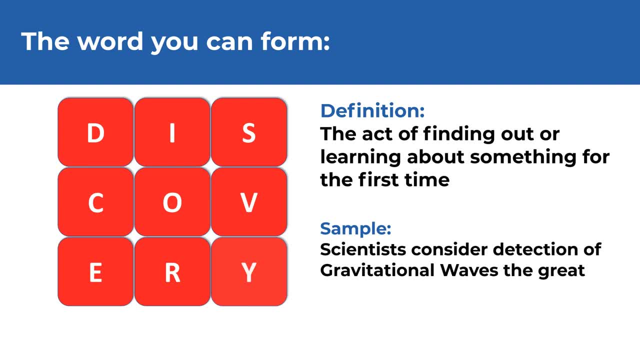 something for the first time, And it is known as the greatest discovery of the 21st century. Did you discover any other words? Make sure to post them in comments And, if you are getting ready for the test and looking for additional questions to practice, 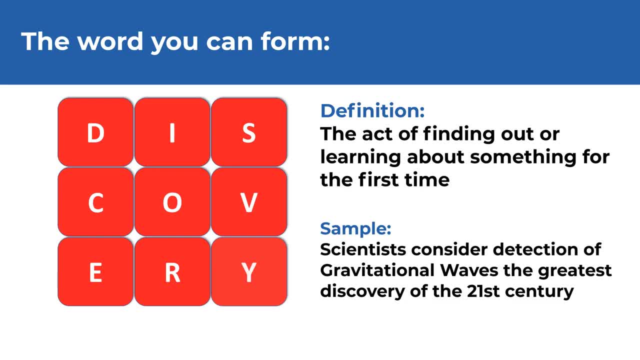 make sure to check the description of this video for links to additional resources. Thanks for watching. If you liked the content, please give us a like and consider subscribing. Thanks for all your endorsement, support and patronage. For additional helpful information, please make sure to subscribe to our channel. 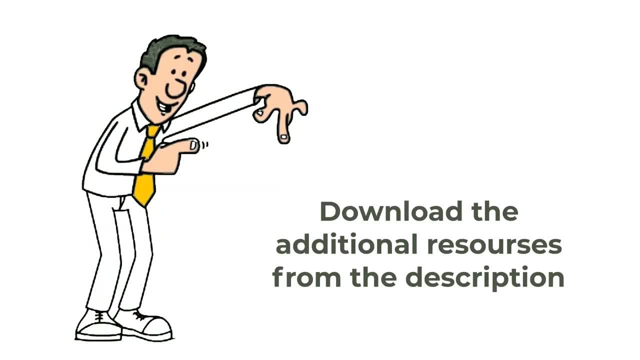 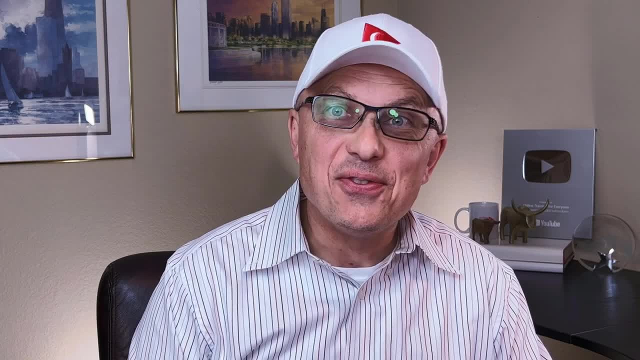